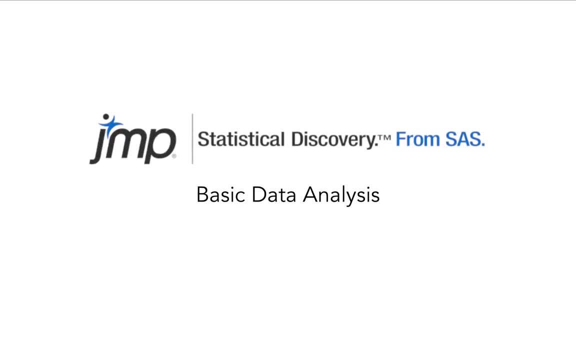 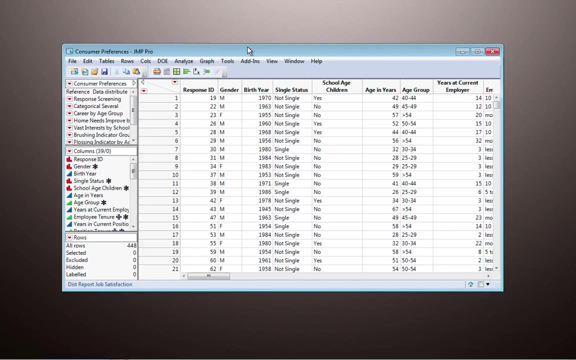 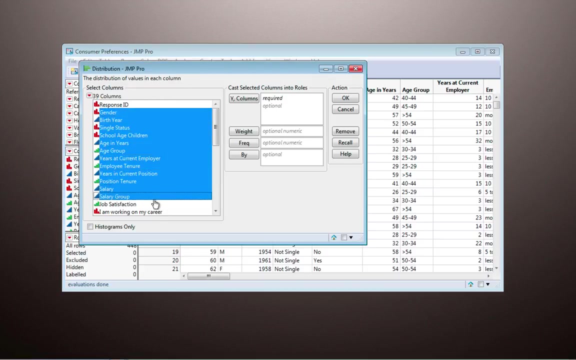 Employing basic tools for visual analysis is often the best way to communicate results and to motivate action. Frequently, your first step in a statistical data inquiry consists of investigating variables one at a time, a process known as univariate analysis In JMP. once we know which columns we're interested in, the distribution platform allows us to. 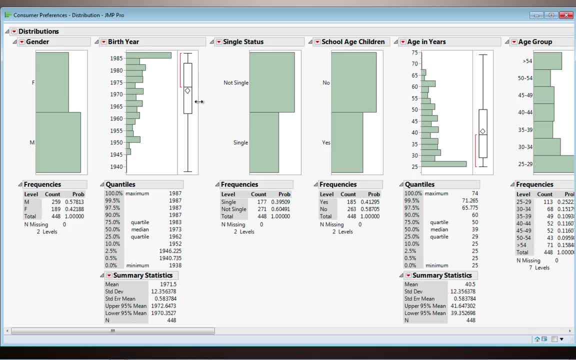 investigate the univariate characteristics of all of our columns at once. Notice here that JMP has produced output that is sensible for the types of variables we have. For our continuous variables, JMP has produced proper histograms and quantiles and summary statistics. For our categorical variables, JMP has produced frequency distribution plots and frequency. 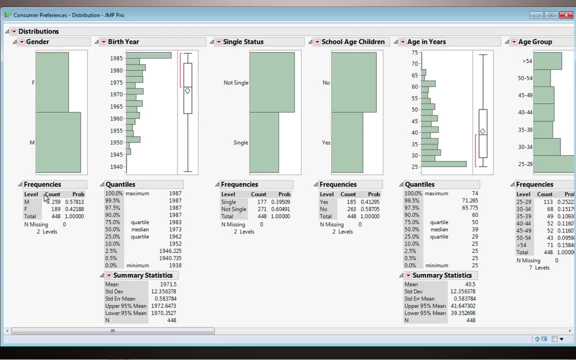 tables. Like all platforms in JMP, once we've produced an analysis, we can continue to dig deeper. The red triangles next to our continuous columns give us the option to analyze the distribution of all of our columns at once. The red triangle gives us the option to produce normal quantile plots or to test a mean or 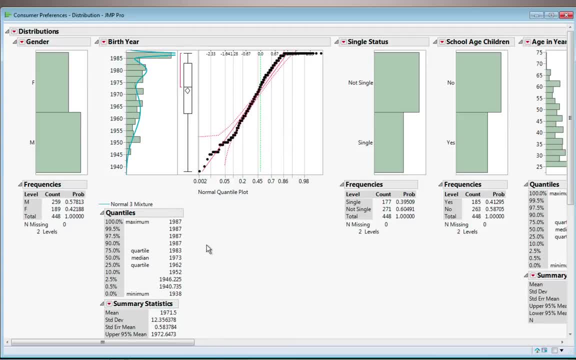 even to fit continuous distributions. We can fit all of them at once here and investigate the fit criteria to see which of our distributions fit best. Next to our categorical columns, those red triangles will display different options, because JMP knows that different operations are permissible when we're working with categorical data, Even though the distribution 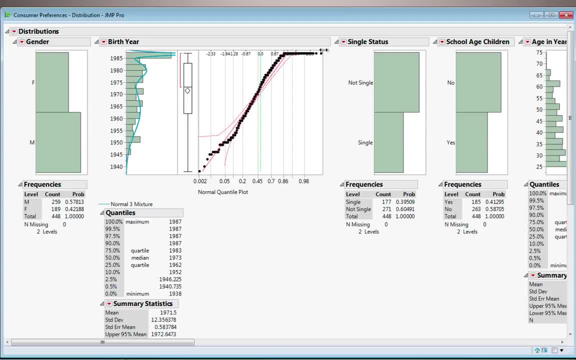 platform is built for univariate analysis. because of JMP's global selection, I can investigate bivariate questions right here in the distribution platform By selecting a category under one of my categorical variables. we can see all those observations in the other platform outputs. 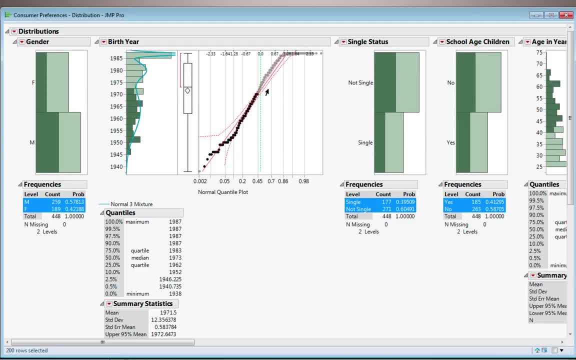 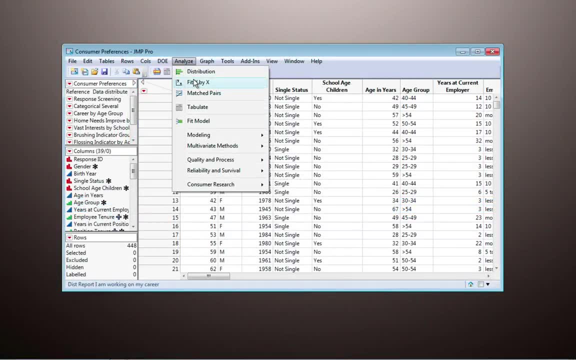 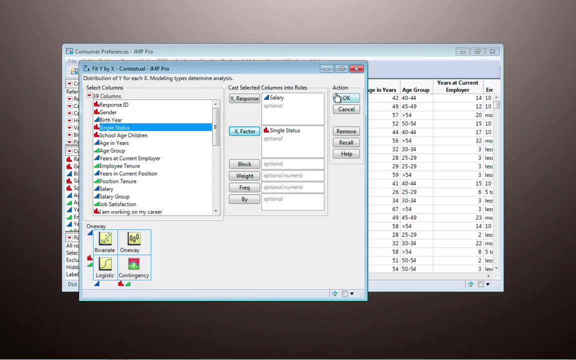 I could also select observations in my continuous columns and see where those observations are in the other plots. For formal bivariate analyses we'll go to the fit-y-by-x platform. The fit-y-by-x platform, just like the distribution platform, is sensitive to the type of variables you 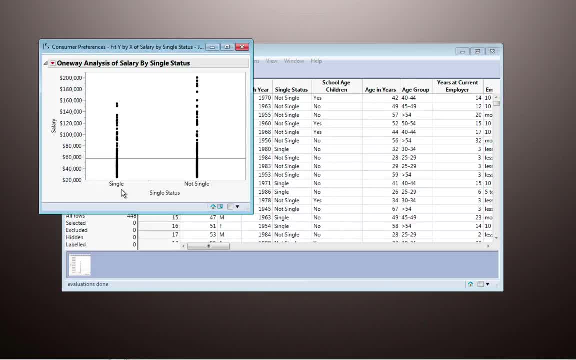 provide. As students trying to identify the conditions for anatomical analysis, we find that the distribution- So here, when I'm predicting something continuous on the basis of something categorical- Jump knows to provide me options like an ANOVA and a pooled t-test. 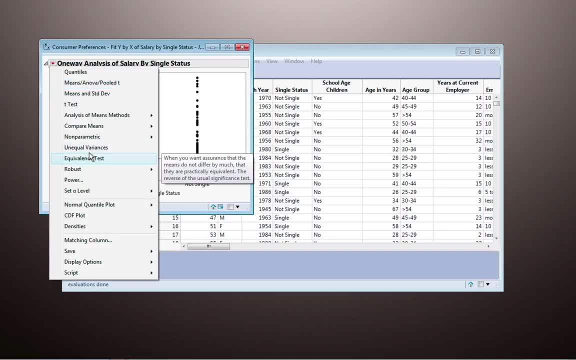 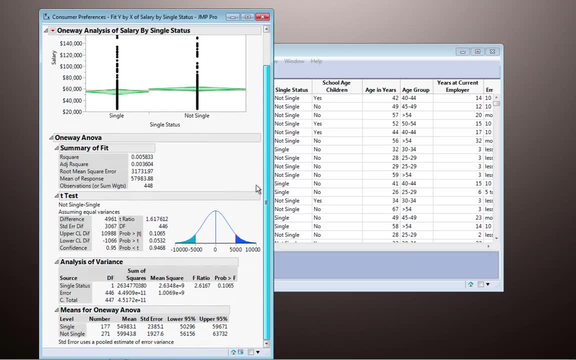 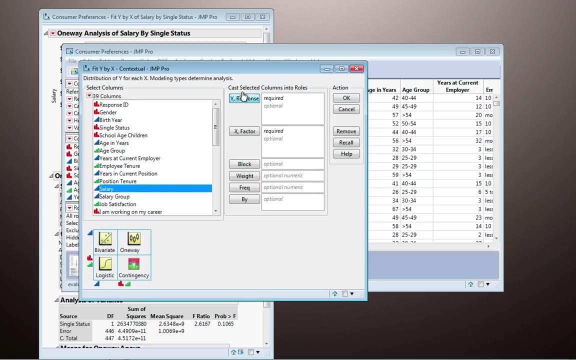 or comparing for unequal variances or performing an equivalence test. All of these analyses will be produced inline, so simply by clicking. the output is shown in the window we already have open. Jump knows that if I specify different variables, perhaps a continuous variable, I'm predicting on the basis of another continuous variable.